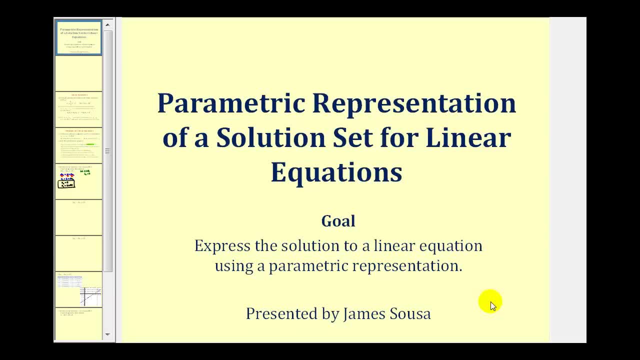 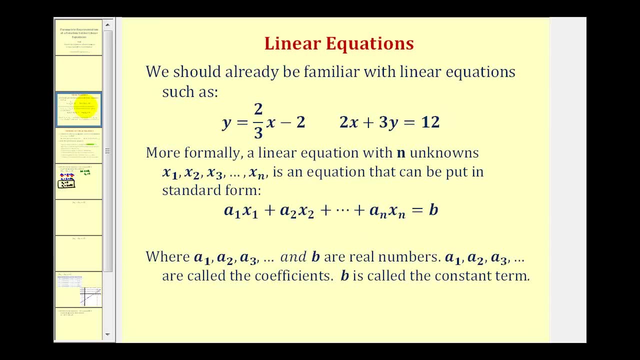 Welcome to a lesson on the parametric representation of a solution set for a linear equation. We should already be familiar with linear equations in the form of, let's say, y equals 2 3rds x minus two, which is a sloped intercept form of a line. 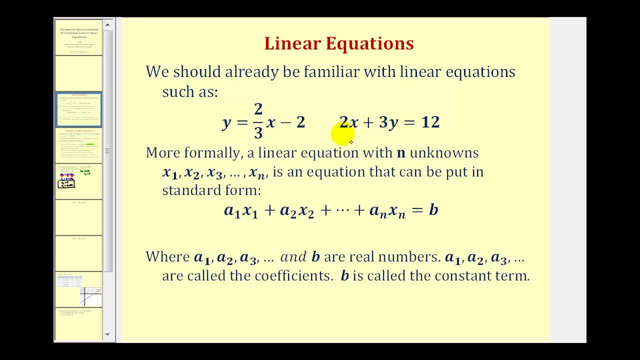 as well as two, x plus three, y equals 12, which is the standard form of a linear equation. But to define a linear equation more formally, a linear equation with n unknowns, x sub one, x sub two, all the way through x sub n. 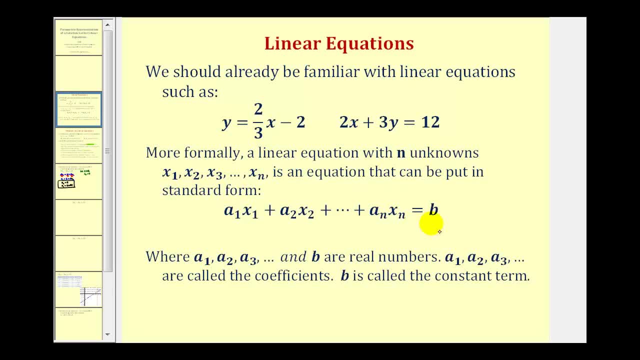 is an equation that can be put in standard form or this form here, Where x sub one, x sub two all the way through, x sub n and b are real numbers. the a's are called the coefficients and b is called the constant term. 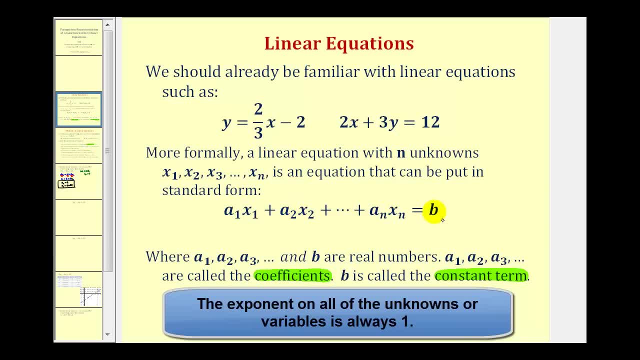 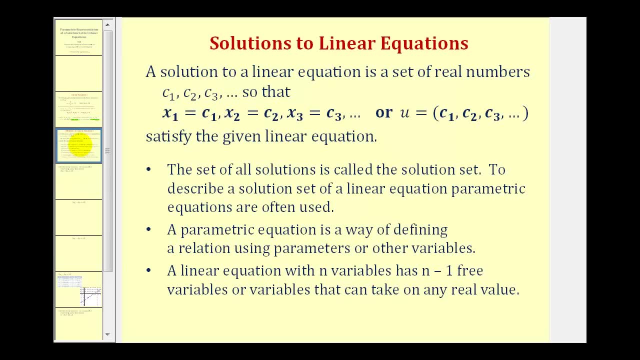 Notice the a's are being multiplied by the unknowns and b is the number without the variable. A solution to a linear equation is a set of all real numbers: c sub one, c sub two and so on, such that x sub one equals c sub one. 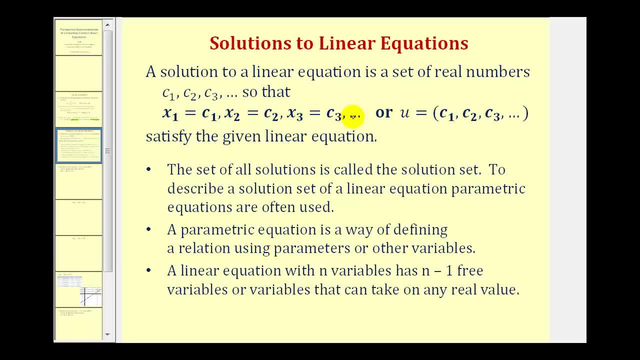 x sub two equals c sub two, x sub three equals c sub three, and so on, satisfy the given linear equation. The set of all solutions is called the solution set, and to describe a solution set for a linear equation, parametric equations are often used. 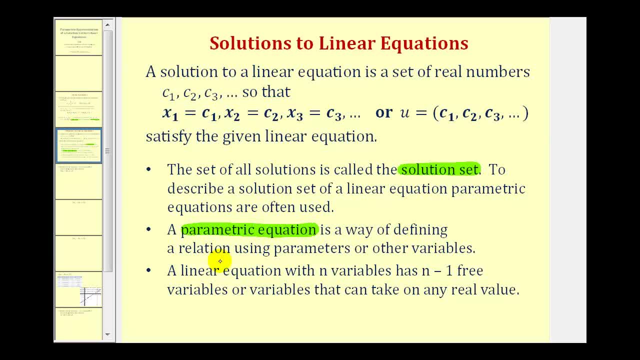 A parametric equation is a way of defining a relation using parameters or other variables. And then, finally, a linear equation with n variables has n minus one free variables or variables that can take on any real value, which will assign the parameters or other variables to. 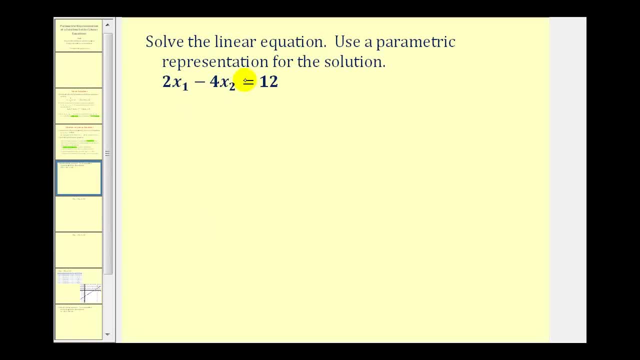 Let's take a look at an example. We want to solve the linear equation and use a parametric representation for the solution. We have: two times x sub one minus four times x sub two equals 12.. So the first step is to solve this for x sub one. 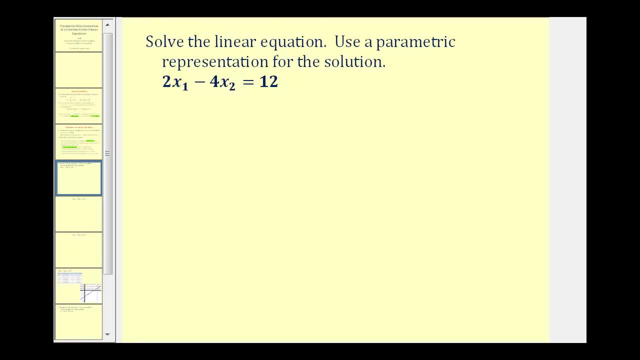 or x sub two. Let's go ahead and solve this for x sub one. So our first step is to add four times x sub two to both sides of the equation. That would give us two times x sub one equals 12, plus four times x sub two. 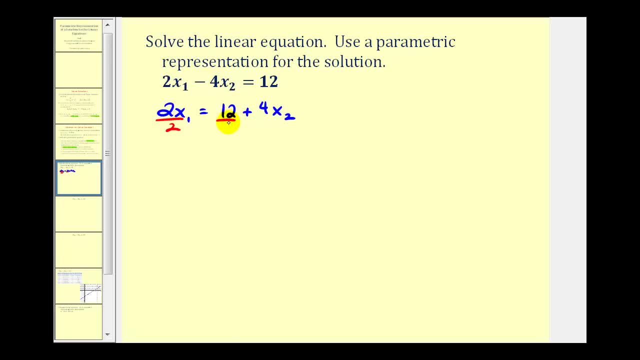 Now let's go ahead and divide everything by two. So now we have: x sub one equals six plus two times x sub two, Because we have two unknowns and one equation. we have one free variable, So we should recognize that we are going to have 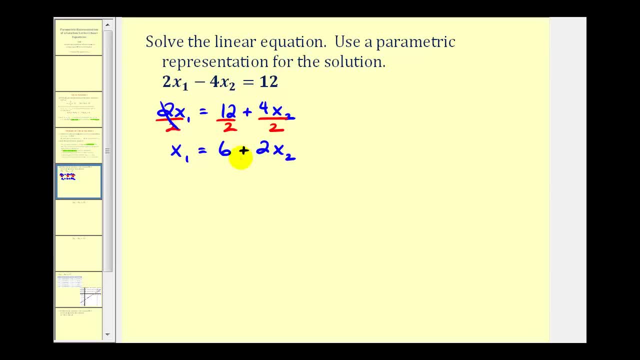 an infinite number of solutions And because of this, we'll introduce a third variable or a parameter which we'll assign to our free variable. Let's let x sub two to be our free variable. Let's also let t be any real number. 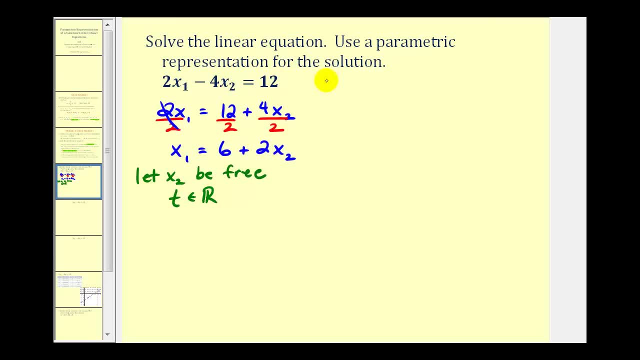 And since we're letting x sub two be our free variable to represent our solution parametrically, we're going to let x sub two equal t, which means x sub one would have to be six plus two times t, replacing x sub two with t. 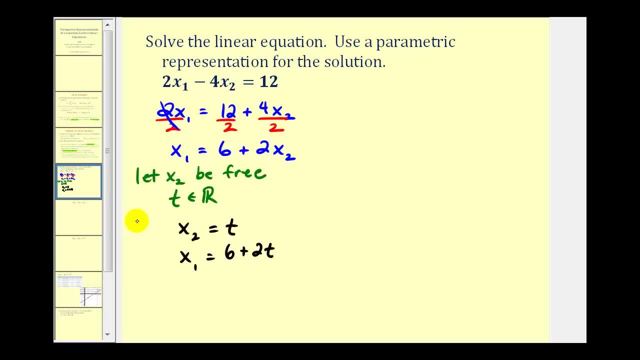 So this is one way to represent the solution to our linear equation parametrically. And I say one way because the parametric representation of a solution is not unique. So just to illustrate this, let's say we let x sub one be our free variable. 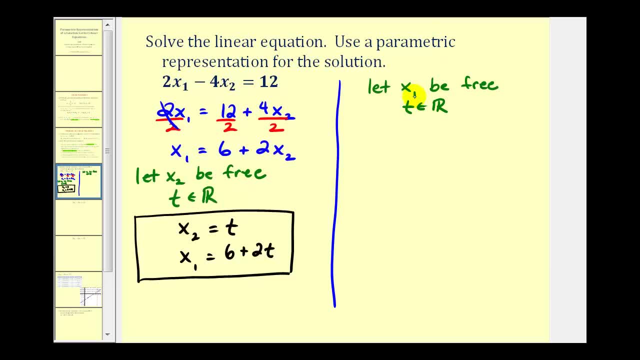 And again we let t be any real number, But in this case, to form our parametric representation, let's let x sub one equal t And therefore, using this equation here, the second equation would be: t equals six plus two times x sub two. 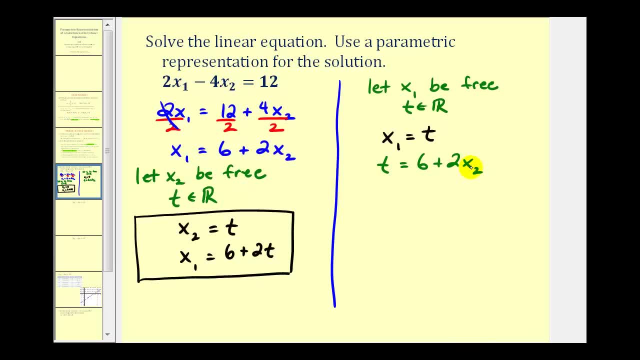 And now we'd have to solve this equation for x sub two. Let's go ahead and do that. We subtract six on both sides. That would give us t minus six equals two times x sub two. Divide everything by two. We'd have one half. t minus three equals x sub two. 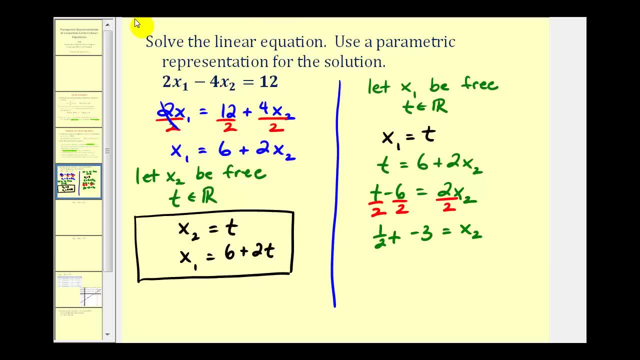 So we could represent the same solution parametrically as x sub one equals t and x sub two equals one, half t minus three. These are two different ways to represent the solution parametrically. Often in algebra class we are asked to graph: 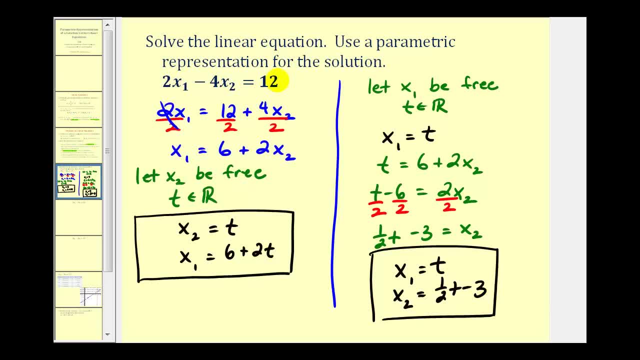 our linear equations, and we could do the same here using the parametric equations rather than the original equation. Let's go ahead and do that using the solution expressed, using the solution Using these equations here. So we'll make a column for t. 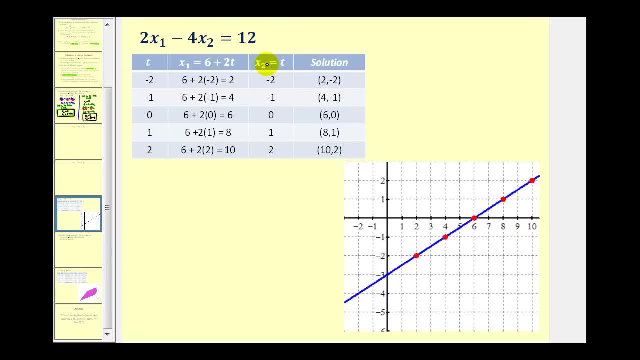 which can take on the value of any real number, And we have x sub one, and then we have x sub two. Well, the first thing we should recognize is that whatever t value we select, it's also going to be the value of x sub two. 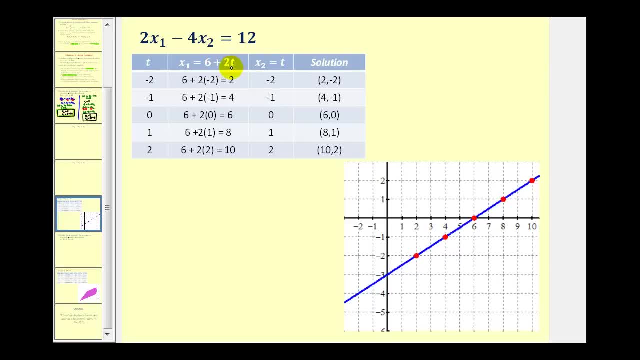 And then, since we know that x sub one equals six plus two times t, we could substitute the same values for t to get the values for x sub one, Every x sub one and x sub two forms ordered pair, which represents one possible solution. 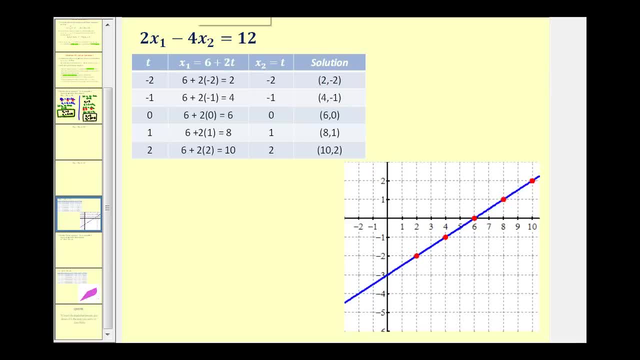 which we can graph on the coordinate plane, Again thinking of the x-axis as the x sub one axis and thinking of the y-axis as the x sub two axis. If we plot these five points, we can sketch our line, which is another way to represent a solution. 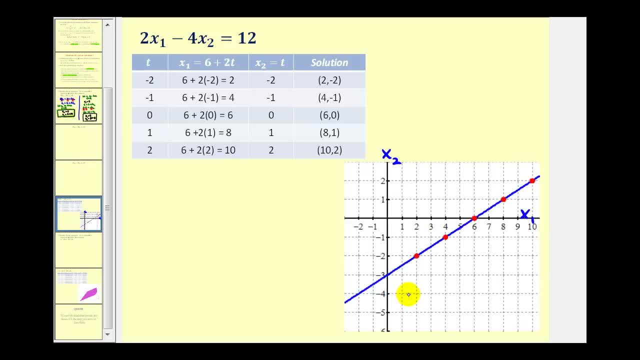 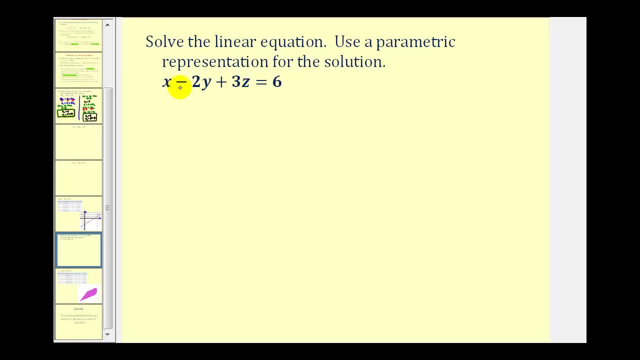 to a linear equation with two unknowns. Let's take a look at a second example. Notice: here we have one equation with three unknowns, and three minus one is equal to two. so here we'll have two free variables, which means we'll introduce two parameters. 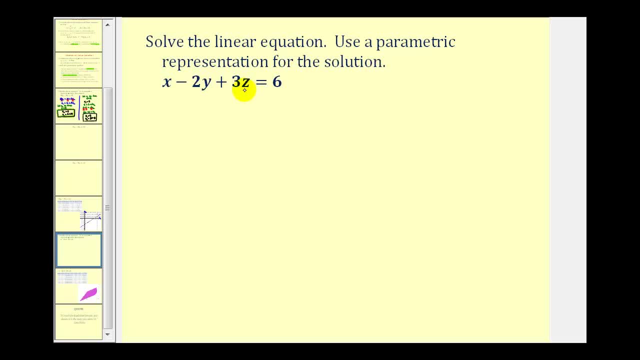 or two new variables to represent the solution parametrically. Looks like it's going to be easiest to solve this for x, so we would add two y to both sides, as well as subtract three z, so we would have x equals six. 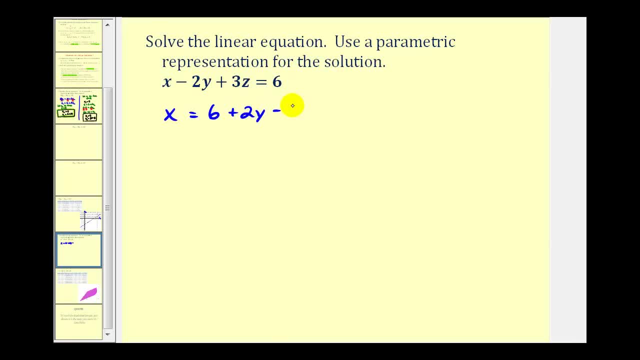 and then plus two y, minus three z. So in this case, let's let y and z be our free variables, so we'll introduce two parameters or two new variables. Let's let s be any real number and t be any real number. 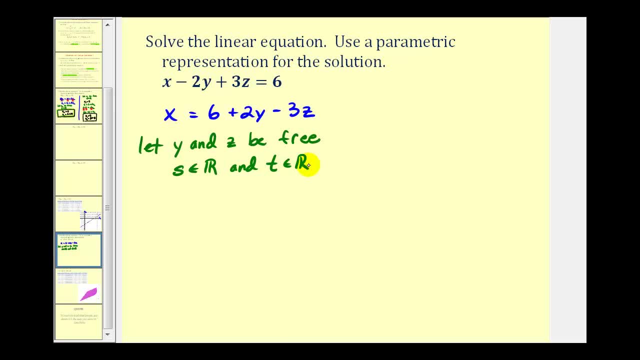 So we'll go ahead and let y equal s and z equal t, which means x is going to be equal to. using this equation here, we would have x equal two and z equal t, which means x is going to be equal to. 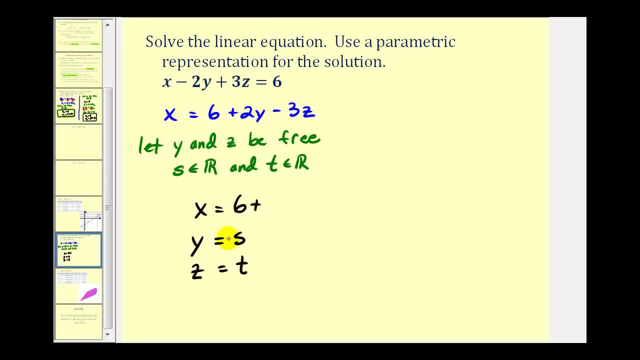 using this equation here we would have six plus two times y, but y is s. so plus two s, minus three times z, but z is t. So this would be the parametric representation of the solution to our linear equation. And because we have one equation with three unknowns, 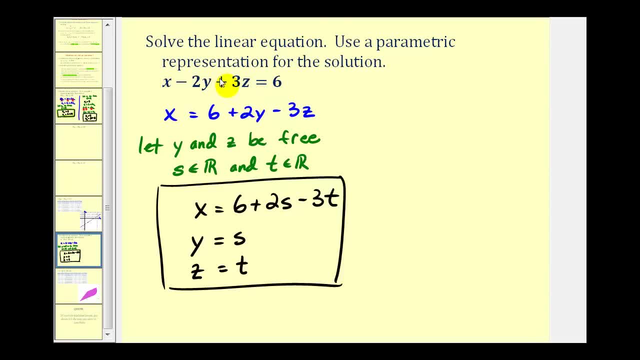 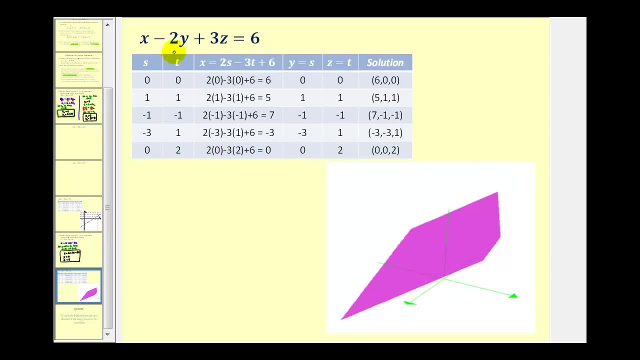 the graph of this would be three-dimensional or it would be a plane in space. Let's go and show how we would do this using the parametric equation. Let's look at the parametric equations Again. we'd start with a column for s and a column for t. 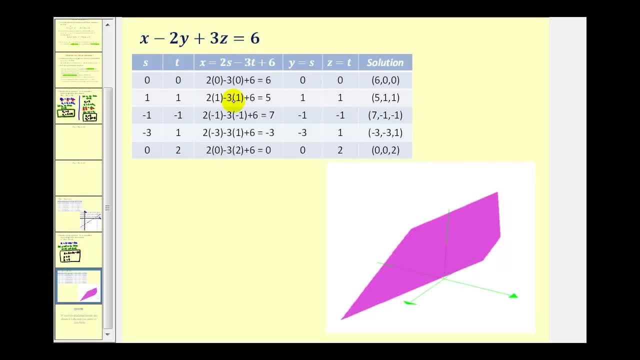 which we'd let be any real numbers. that would be convenient to perform the calculations. and since s equals y, this column and this column are the same. and since z equals t, this column and this column are the same. And then we're left with finding x. 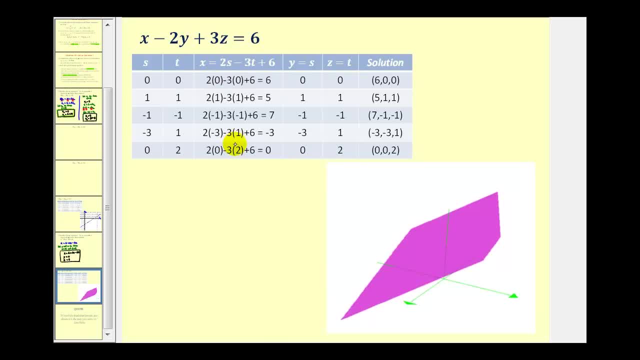 by performing substitution for s and t, which has been done here. Notice, here each solution consists of a value for x, y and z. so we have ordered triples, which would be points in space, which, as we see here, would be a plane graphed in space. Okay, I hope you found this helpful. 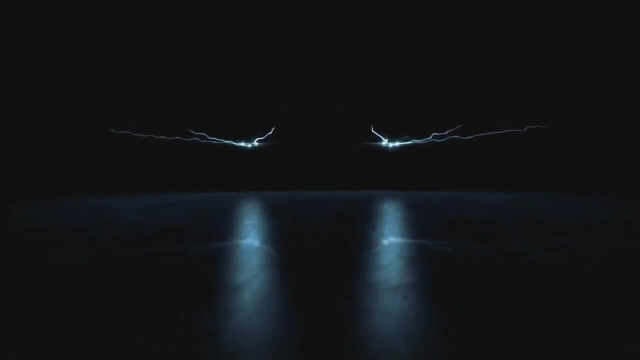 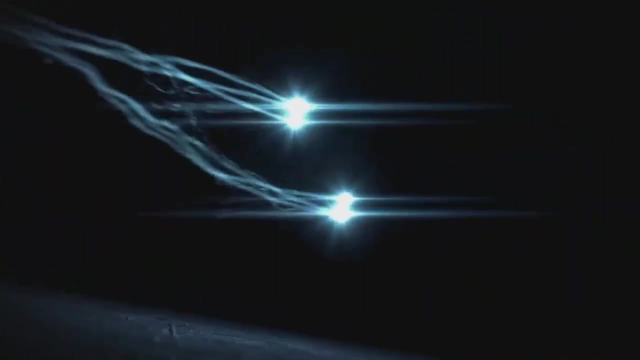 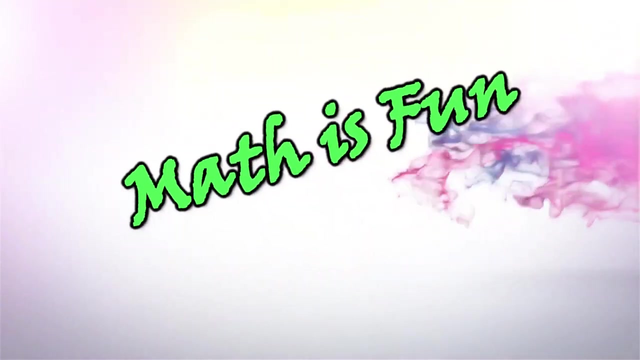 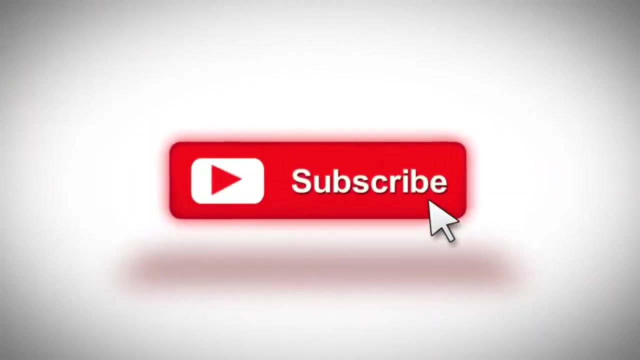 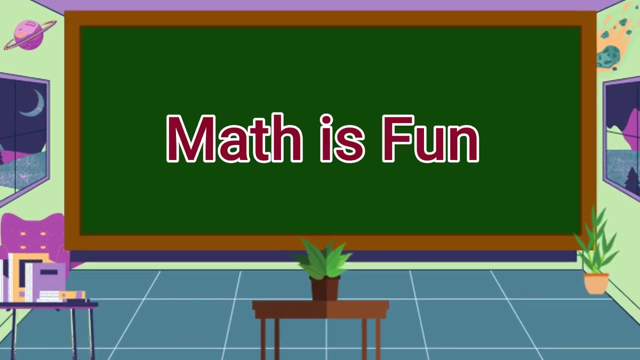 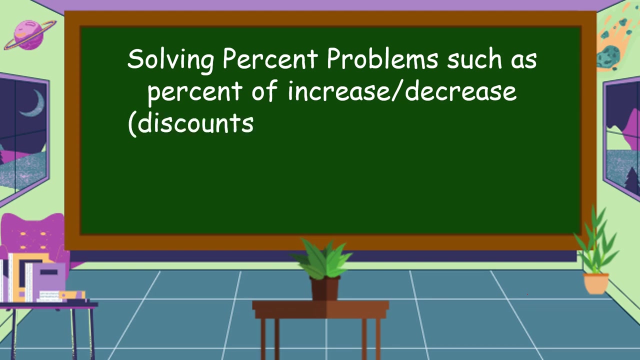 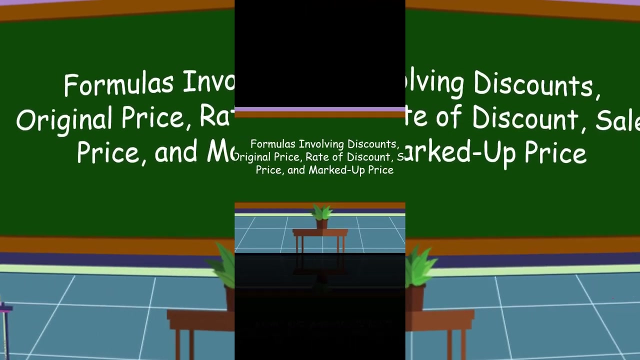 Thank you for watching. Hello everyone, welcome to Must is Fun. Our lesson for today is all about solving percent problems such as percent of increase or decrease discounts, original price rate of discount, sell price and markup price. I'm going to share with you the formulas involving discounts: original price rate of discount, sale price and markup price. 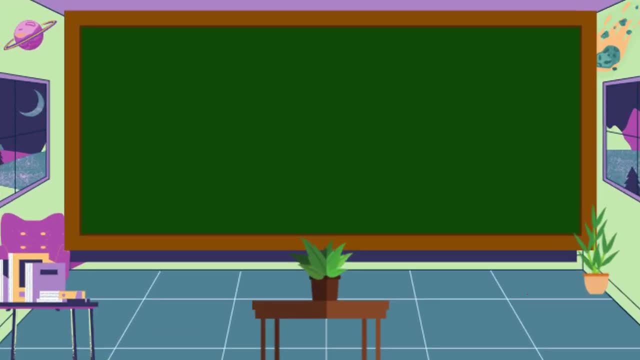 Here are the formulas. If we're going to find the amount of discount, our formula is: amount of discount is equal to original price or markup price times discount rate. If we're going to find the original price, our formula is: original price is equal to sale price divided by 100% minus discount rate.